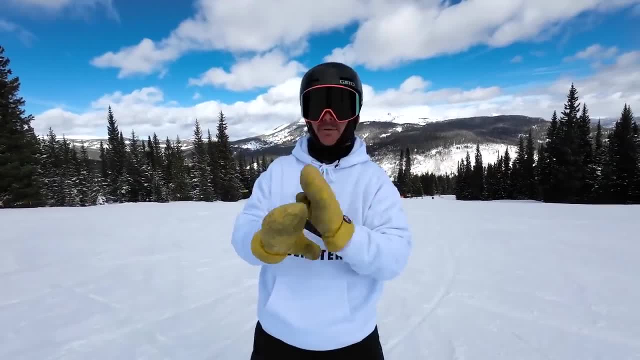 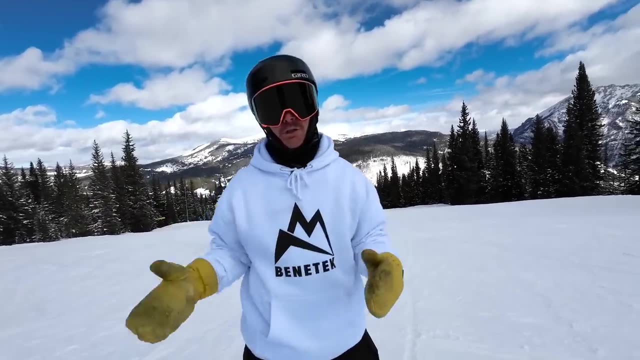 Now you may be asking why or where would I actually use this technique, And I would say you use it 90% of the time as long as you're not carving. So if you're in the trees, you're in the moguls, you're on street terrain, mellow terrain, you can use this tactic. 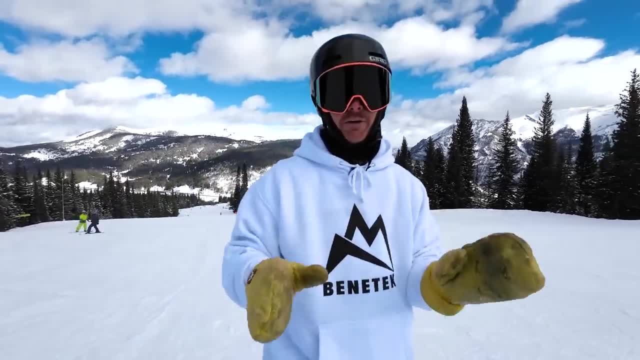 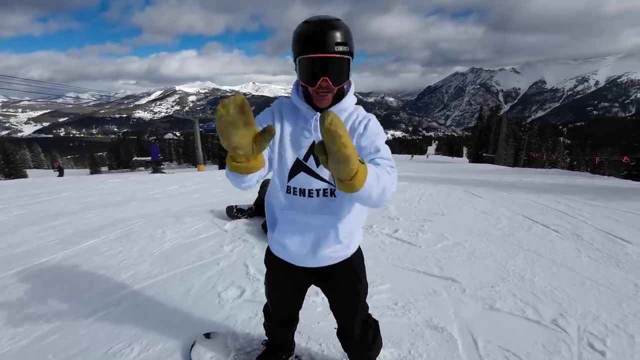 And then if you're carving. it's a little bit of a different tactic, but you definitely want to use this, And you can even use this when you're riding switch, which is even more amazing. So in this video, I'm literally going to break it down step by step by. 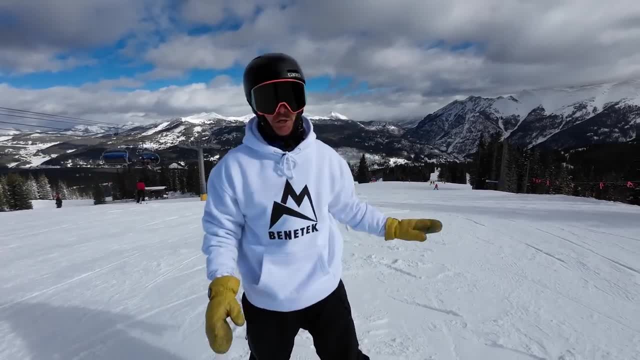 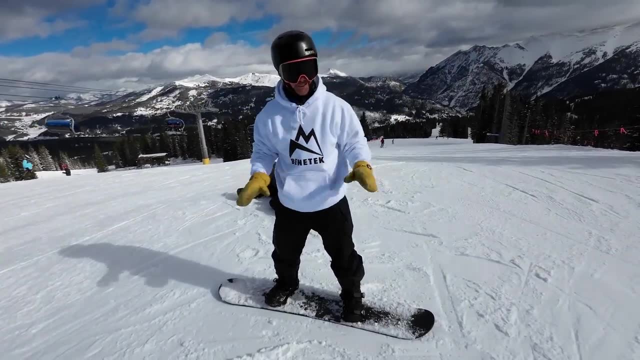 step. So if you want to follow along at home or the next time you go snowboard, we're definitely going to be breaking it down. So we're going to start off by being in a static position, which means find a nice area where your board can stand the snow and you're not going to move. 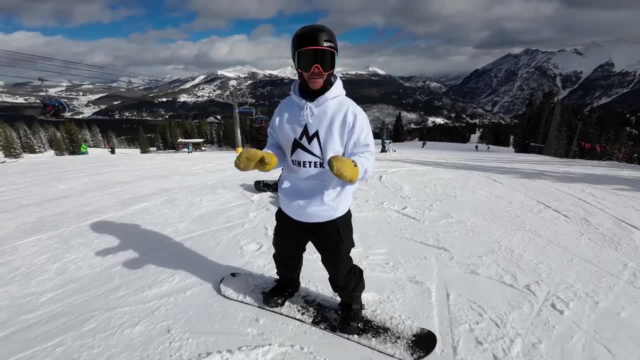 around. We're going to first identify our toe side edge, because I feel like that's a little bit more challenging, So we're going to identify that first. then we're going to break down our heel side, So our toe side edge is going to be a little bit more challenging, So we're going to 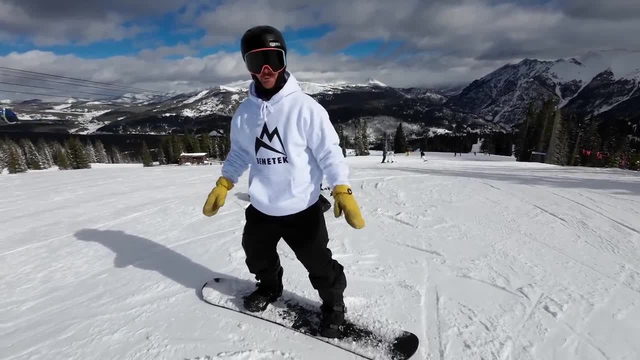 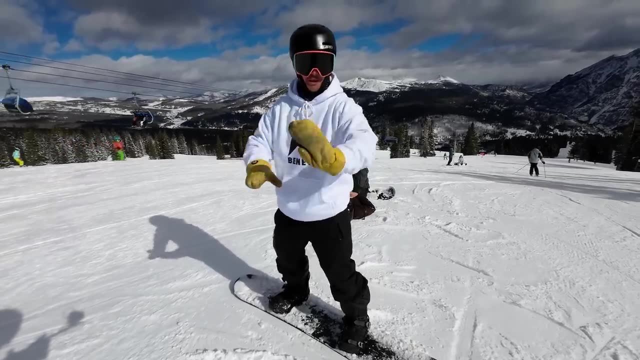 When you're strapped in, whether you're regular or goofy, what I want you to think about is keeping your shoulders, hips and knees stacked over your toes in a nice athletic position. Now, whether you're regular or goofy, the only thing in theory should change is just where we are. 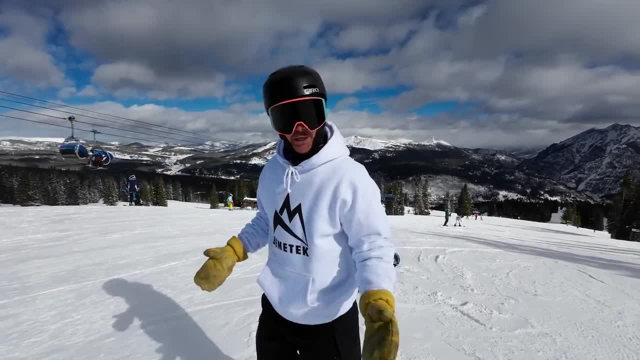 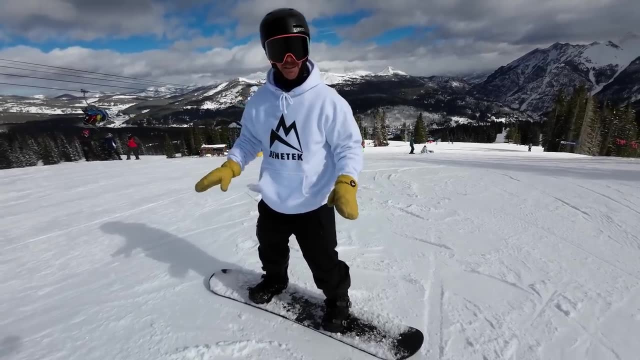 looking. So now for this example. I'm a regular rider And so what I'm doing is I'm facing uphill and I want to shift about 60% of the weight into my lead foot. As I'm in this position, I'm mimicking this as we do our next step, So remember. 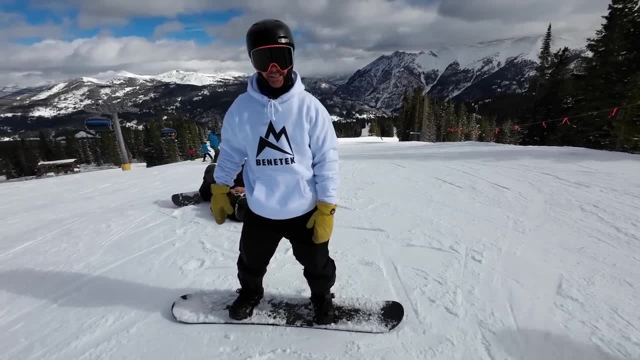 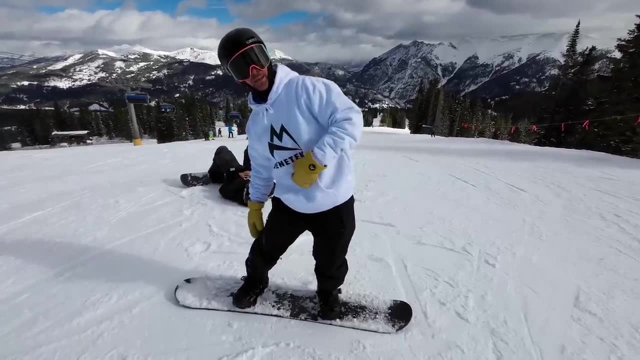 I want to keep my shoulders, hips and knees over my lead binding, And one thing not to do is somebody will try to shift their hip and they do this. Well, technically, my belly button and my balance is over here, but some of my body's there. It's a very contradicting position. 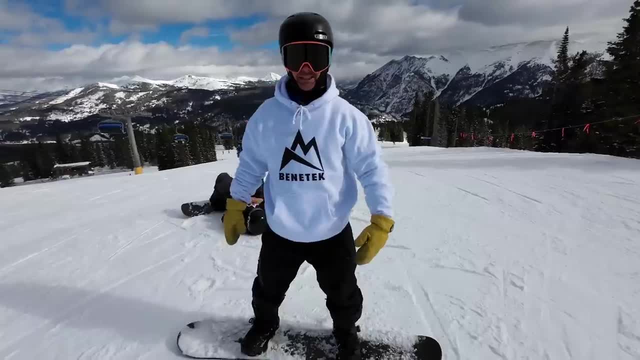 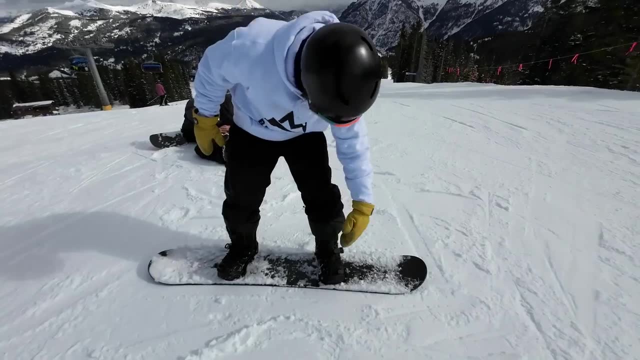 so it's not actually useful. So, shoulder, hip and knee- over that lead binding, I'm in a nice, awesome position. From here, what I want to feel is that my shin is pressing against the front of my boot, as if there's a bug on my heel strap. So I'm going to keep my shoulders, hips and knees. 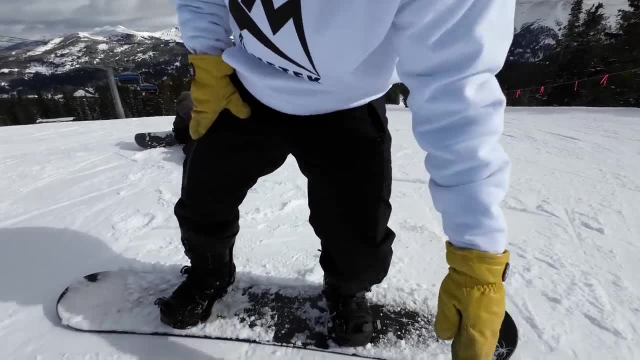 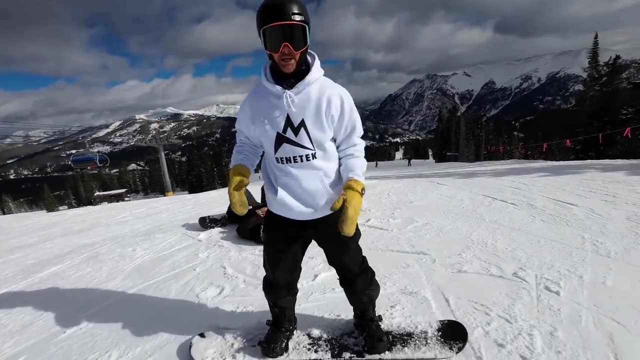 over my ankle strap and I'm trying to press my knee over my toe, just like this, So as I stand up and look from a global view, as you can see my whole body from here, I'm doing this. Notice that. 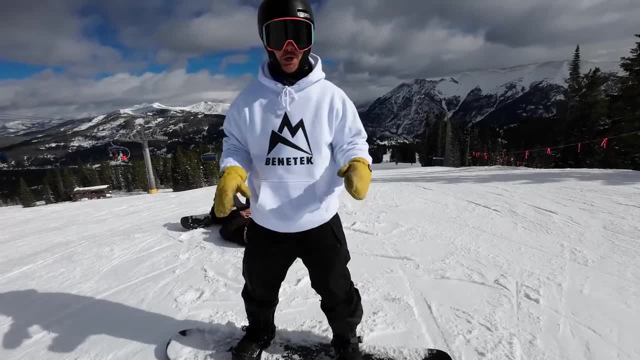 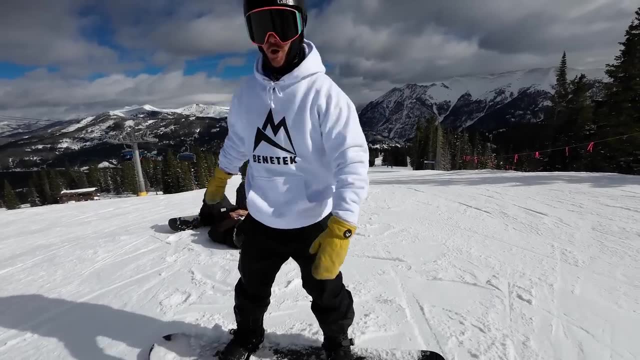 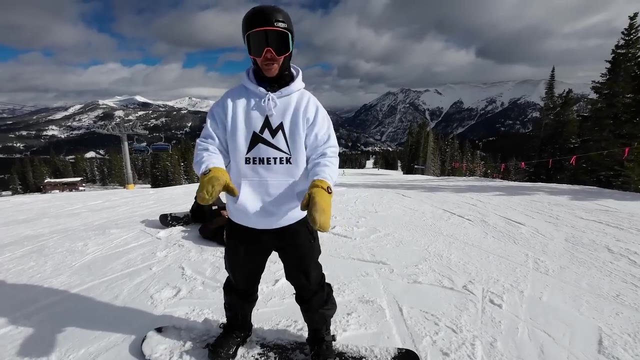 I'm not just pressing my shin and my lead shoulder staying elsewhere. I still have that lead shoulder, hip over that binding- but I'm moving my body together. I am not throwing my shoulder on the ground, My arms are quiet and I'm doing this So, as you're at home or practicing, feel the shin. 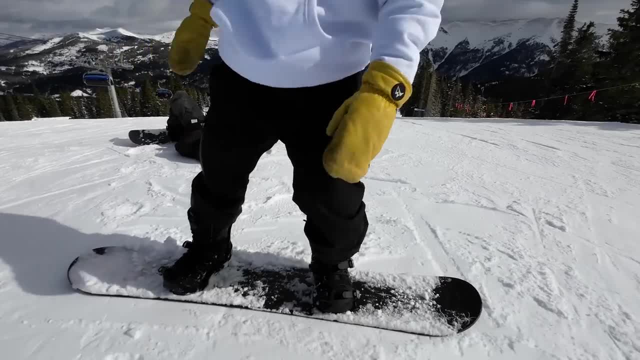 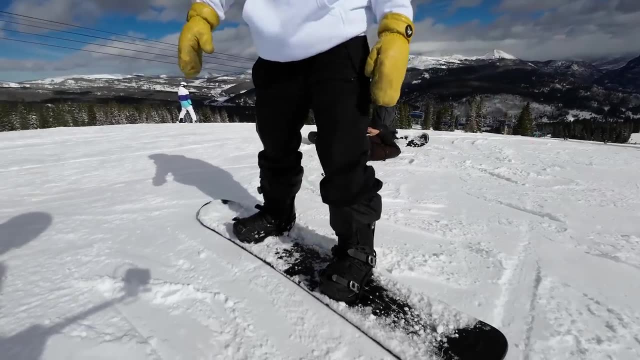 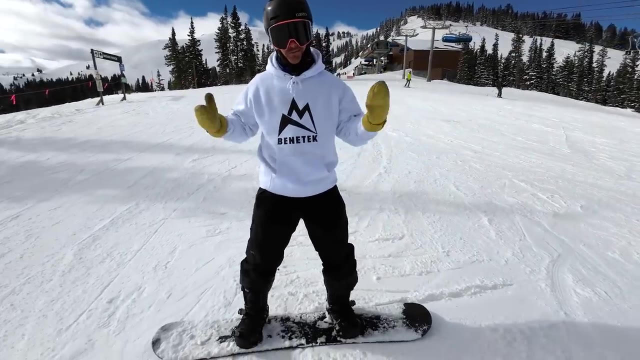 press against the front of the boot 10 times just so you can feel that movement, that engagement, while keeping a look downhill where you're going. So I'm definitively feeling that shin press there. So now let's switch over. For this example, I'm still going to be on my lead foot, which is a 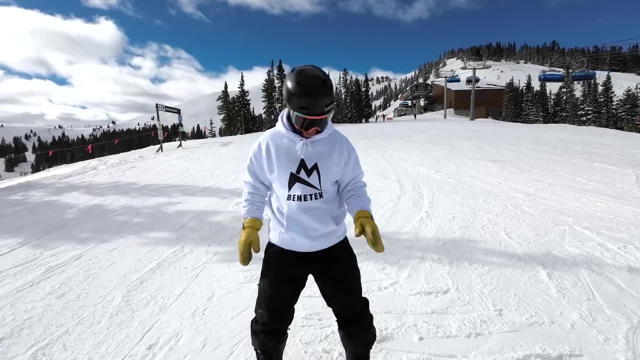 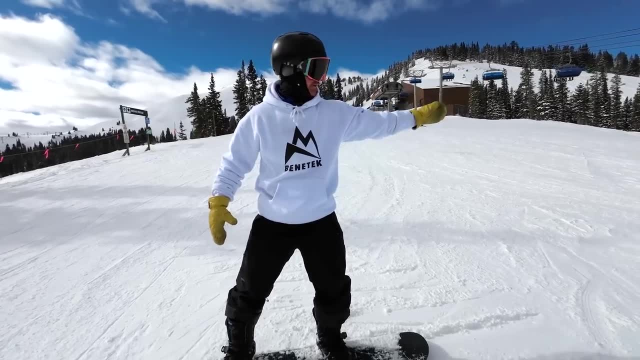 regular rider. Obviously, this still applies if you're goofy or riding switch. So now in this position, I'm once again in a stacked position. 60% of my body weight is on my lead foot, So I'm in this position Now. this time I'm going to kick my hips back just a little bit, but not over. 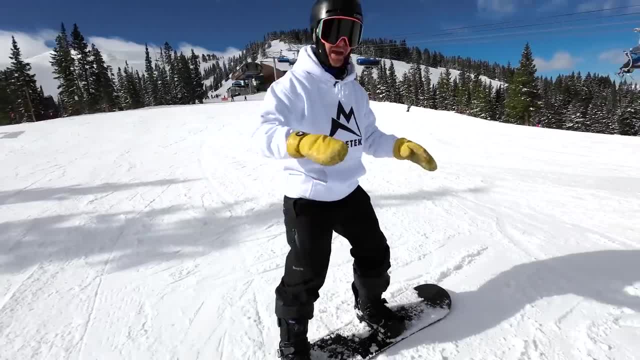 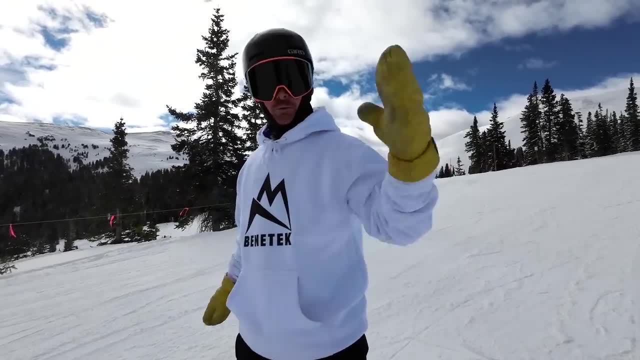 exaggerate where I'm like flexing my spine down, but I'm pushing a little bit back, allowing me to make contact with my high back Now that we have 60% of our weight over our lead foot, which does mean that our shoulder, hip and knee are all stacked over. that binding once again, And I do. 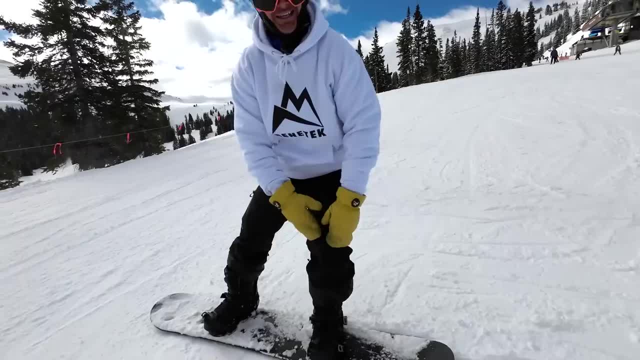 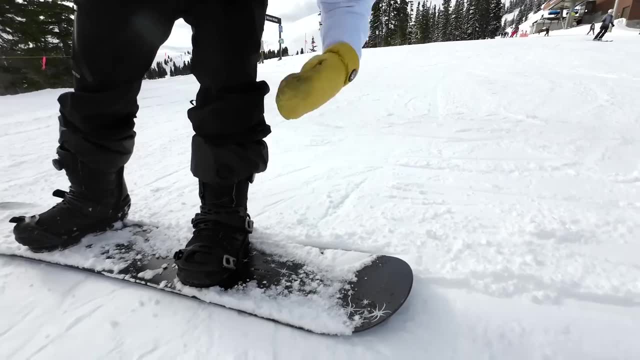 have flexion in my knee From this position. the knee steering actually comes from us rotating our femur to the outside of our board, So I'm almost looking to get my knee to rotate and turn towards the contact point of the board, which means the board starts to rise. That's like. 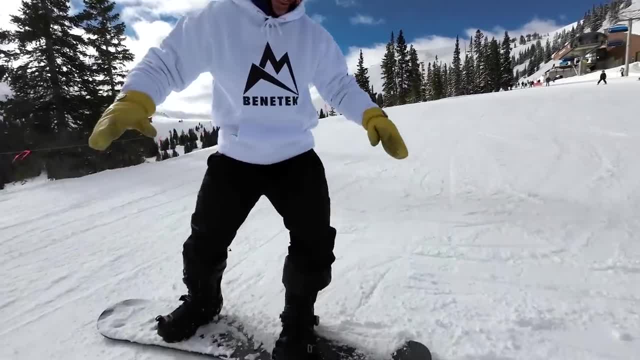 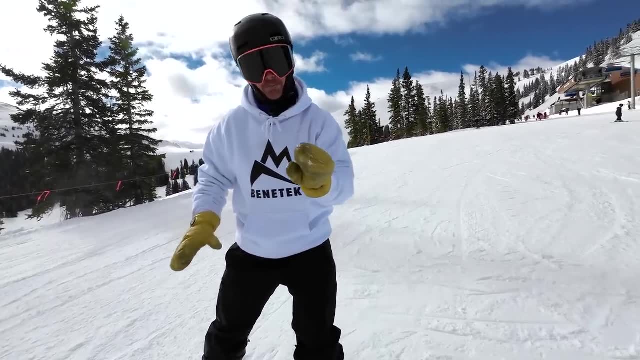 the contact point. So from there I'm here and I'm just trying to push my knee. You're also going to feel that your foot is going to try to rotate within your boot and within the binding And you're putting a lot of pressure on the outside of your heel. Now, that's all what you're looking. 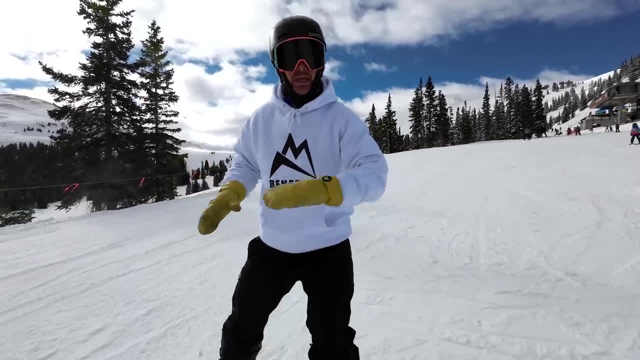 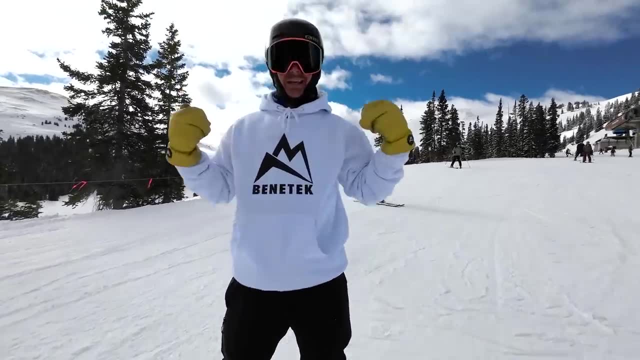 for That's definitely a good thing. So what that's going to do is you're going to be able to rotate your foot, So what that's going to allow us to do is once again pivot that board and get early edge engagement, allowing us to find the balance of me turning in the board turning, And 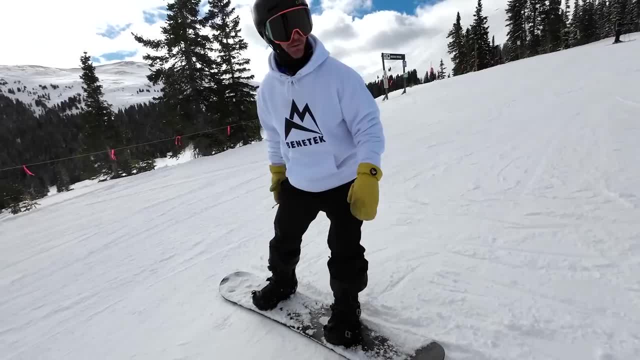 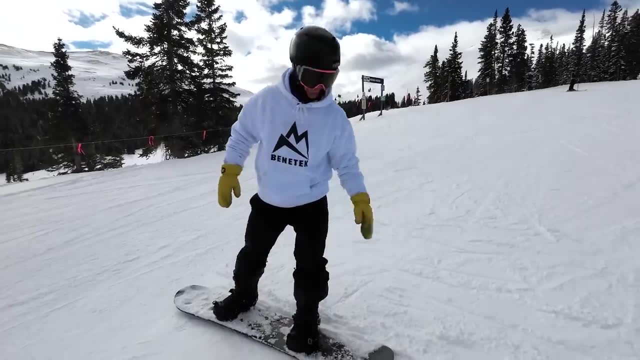 as I do this, I'm trying to keep my eyes up, looking where I'm going, And I'm almost feeling my back foot slightly pivot out. I'm not trying to pivot my back foot, but more rotate that lead foot. So let's go ahead and do that 10 times, whether you're at home or on the slope, And I'm 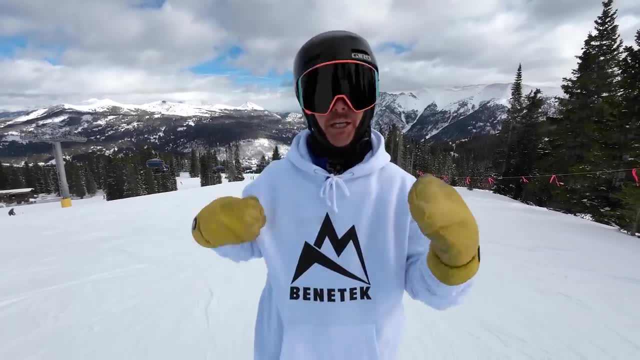 going to interrupt real quick. If you guys are interested in supporting the channel or want to pick up some freaking awesome merch, go ahead and check out shopbenetechcom. So now let's actually start moving and grooving, And this is going to be. 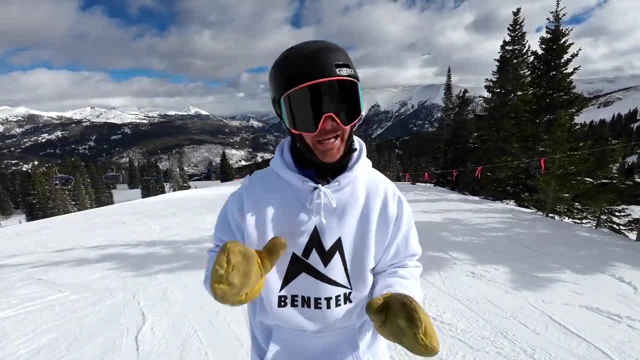 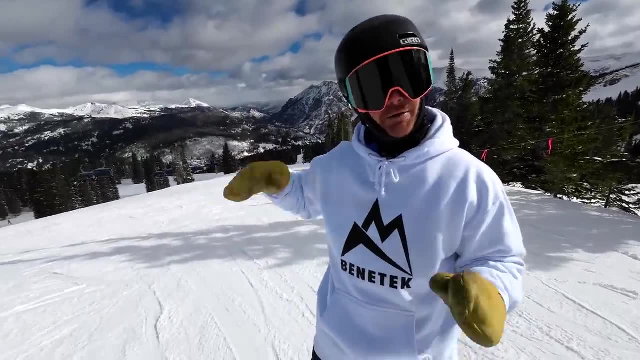 step two. Now we're breaking this up into step A and B, which are going to be our toe side and heel side. So the biggest thing is: you want some sun, Thank you, And you want to find a slope that allows you to point your board straight down the fall line without accumulating a lot of speed. A. 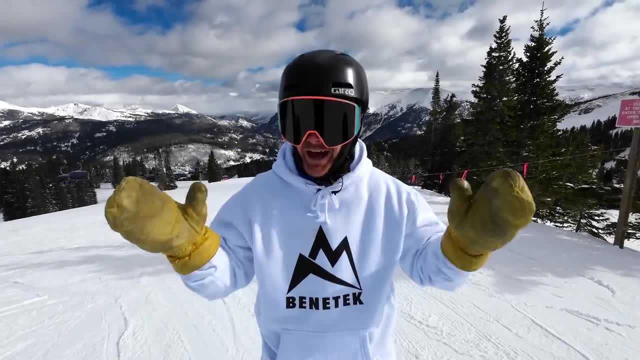 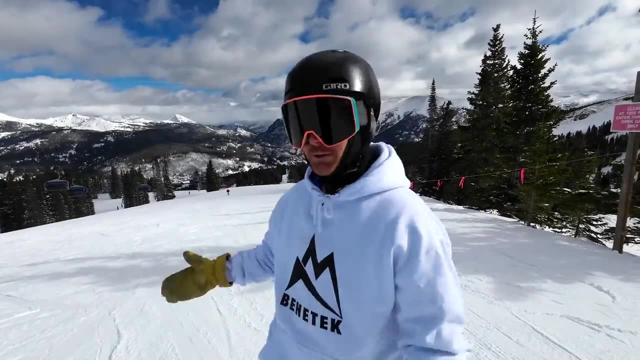 good indication is: can you point your board down the fall line up to five seconds without picking up too much speed and getting uncomfortable? It's definitely a good time If you are more of an advanced rider. finding a little bit steeper slope, totally okay, As long as you're sticking to these body positions. don't get ahead of yourself. 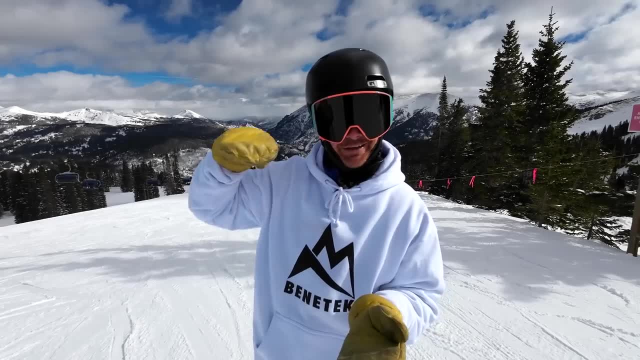 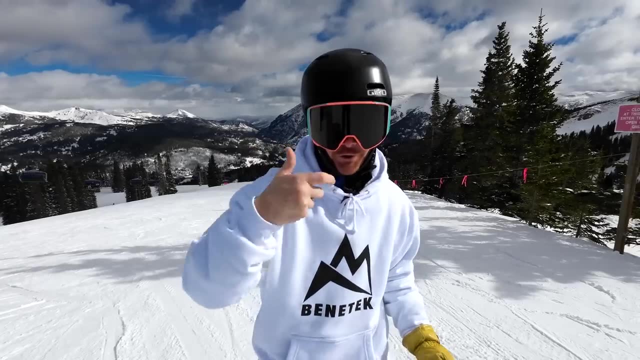 So what we're going to do is the goal is to point our board straight down the fall line. We're going to count to one- 1,000 to 1,000, and then we're going to press our chin over the front of our 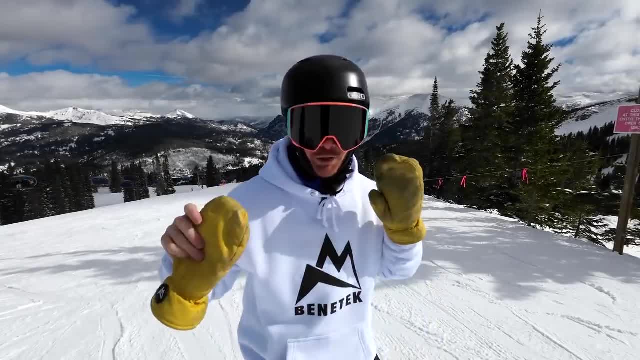 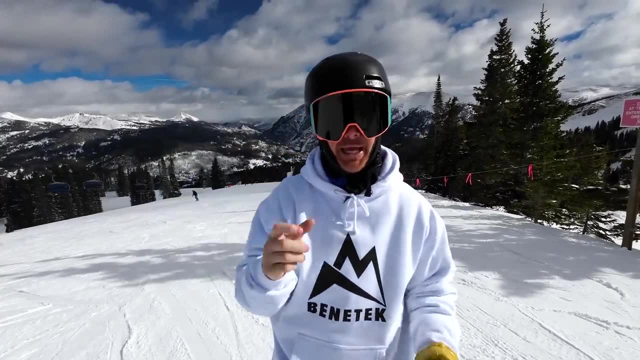 boot Like we did in exercise one. Now what is going to happen is the more aggressive you press your shin, the quicker your board is going to turn. If you gently or progressively press into that, you're going to have elongated but controlled toe side turn. So I definitely 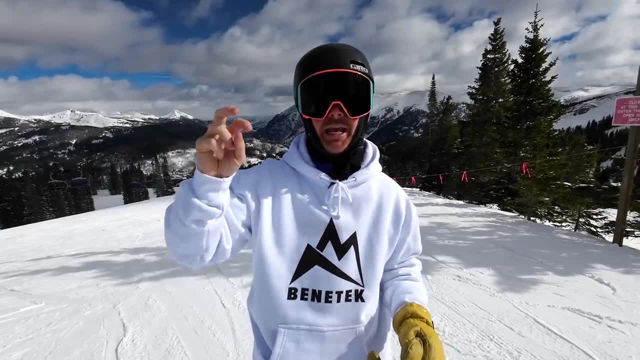 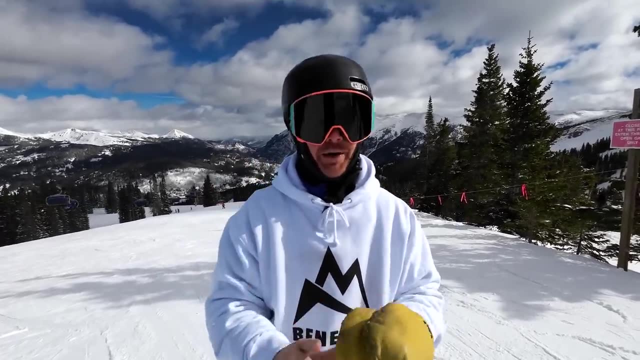 suggest you just feel out both versions, but we're going to start with just a even pressure throughout the shin so that we can feel this. Now you have to be 60% of your weight on that lead foot to allow this to work. If you are in the back seat, this is not going to be awesome. 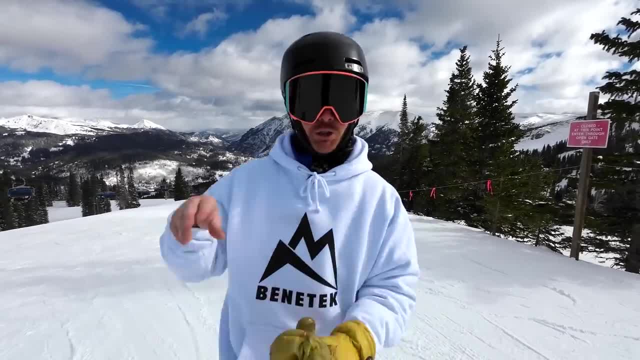 So keep 60% of your weight on the lead foot. Now I'm going to just cruise down. I'm going to show you some visual examples and I'm going to talk through it as we go. Then we're going to break in heel side. Let's go. 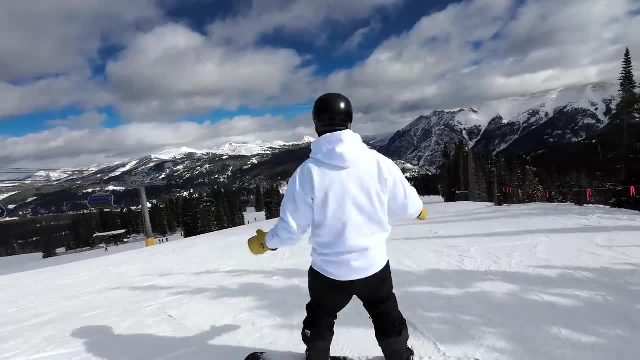 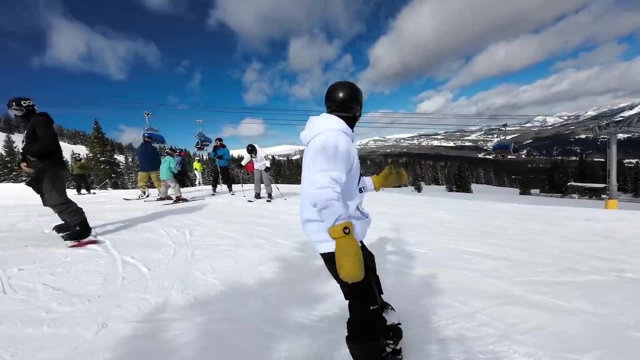 All right. So I'm starting on my heel side edge. I have a nice clear area. I will be looking uphill, making sure it's not too busy. I'm going to point my board down the fall line As I'm pointing my 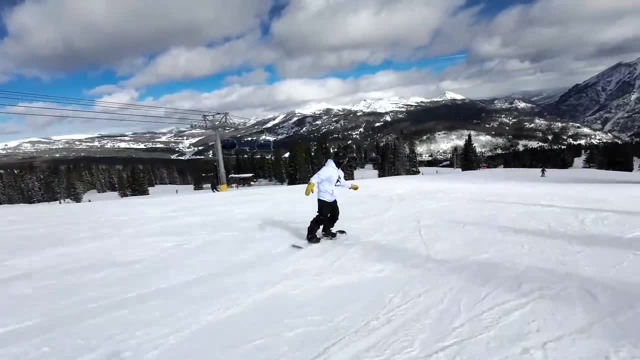 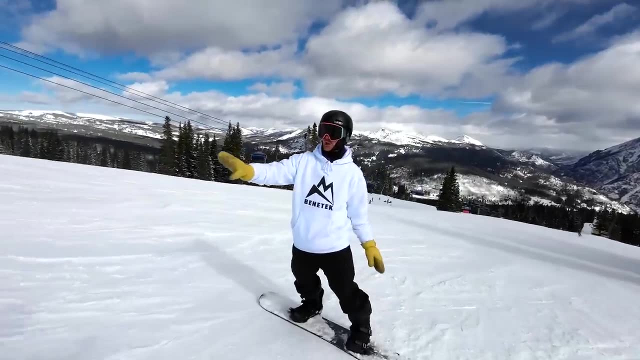 board. down the fall line, I'm getting my weight to be even- One, 1,000 to 1,000, pressing the shin And then, as I get across the fall line, I want to even my weight out. Now, this slope. 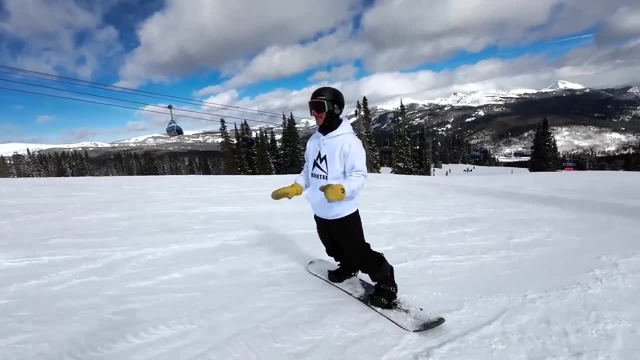 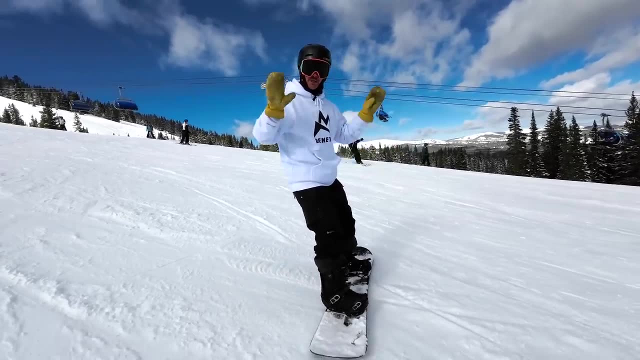 I do accumulate speed a little quickly- That's okay, I'm comfortable with it- but again find the right slope. I'm now going to turn around and I'm going to attempt this five to eight times until I truly feel my shin press against the fur. 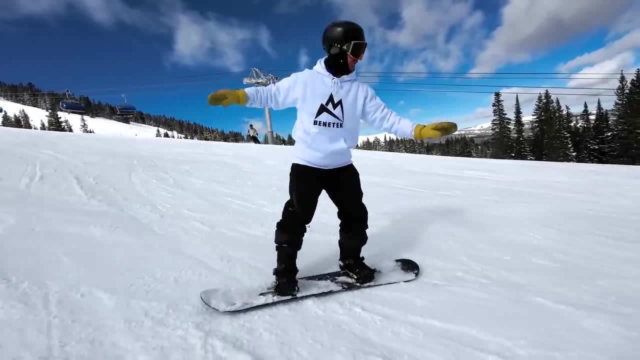 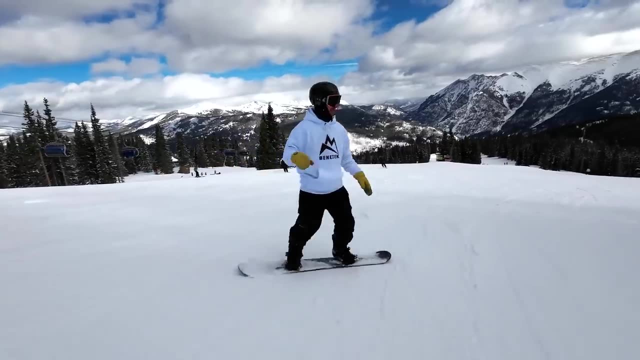 of the boot. Let's go ahead and do it again. Point my board down the fall line, weight forward One, 1,000 to 1,000, press in and then even out. Let's go ahead and do it again. Back to my heels. 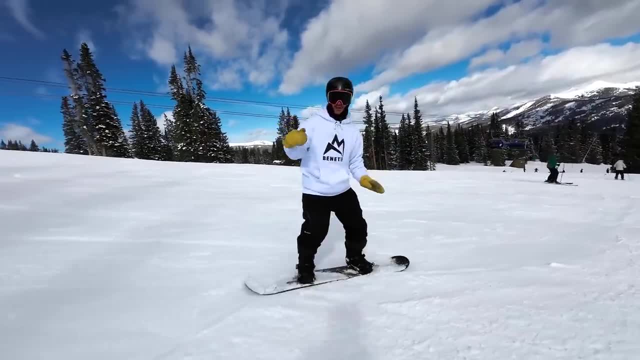 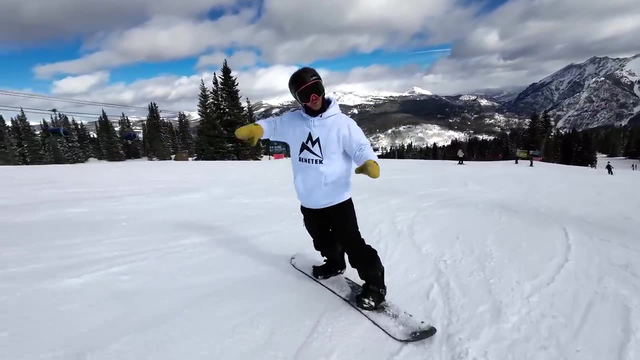 Now, as we do this for the third time, we're going to do this a little bit quicker, just so we can feel that responsiveness. One 1,000 to 1,000 shin Woo Now. did you notice how quickly I 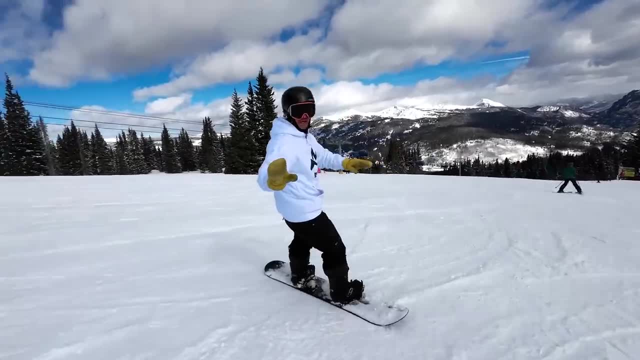 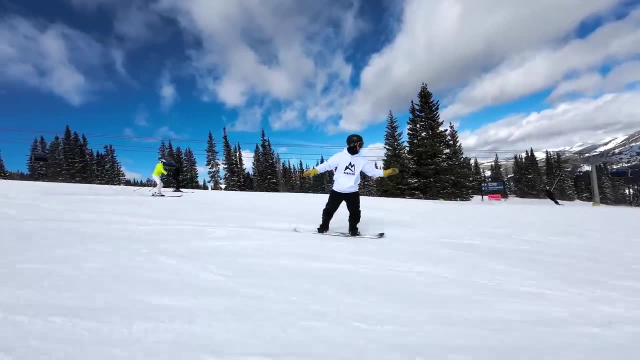 did it. I'm going to do it for the fourth time, but I'm going to be very gentle and see if we can elongate this. So we're going to point our board down the fall line. look around: One 1,000 to 1,000,. 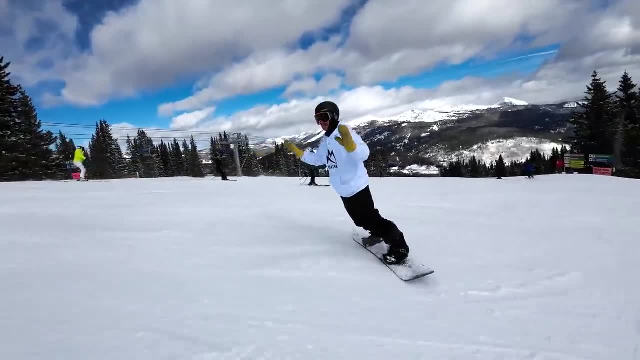 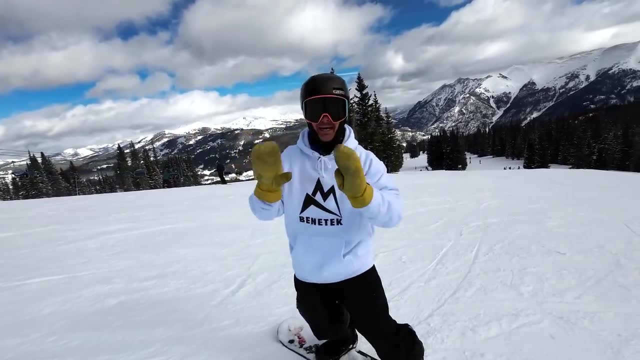 and then I'm going to shin just a little bit, just a little bit, even out Awesome. One good indication that my friend told me big shout out to my friend, who wants to remain anonymous, is: can you pressure shin against your front of your boot while doing this, but wiggle your toes? Now, the biggest thing. 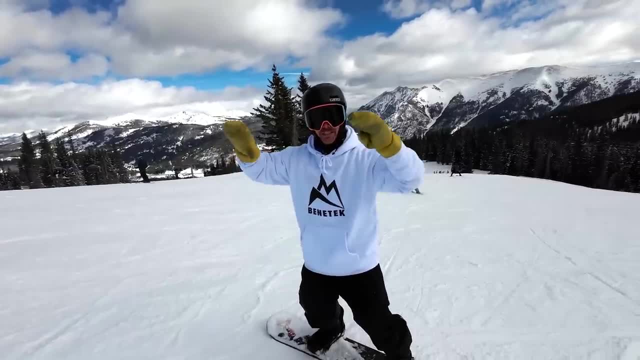 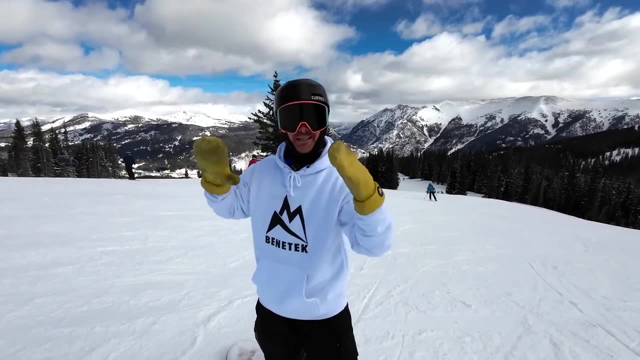 that snowboarders do. that I find to be less awesome is you're actually pressing your toes against the front of your boots and you're gripping down like a hawk and you're trying to grab like your dinner. that's not what we're actually trying to do, because that means that you're doing this. 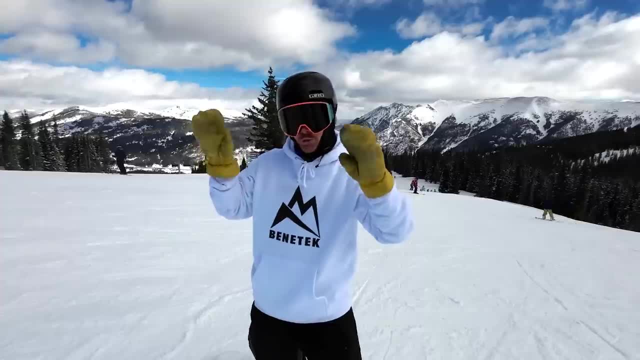 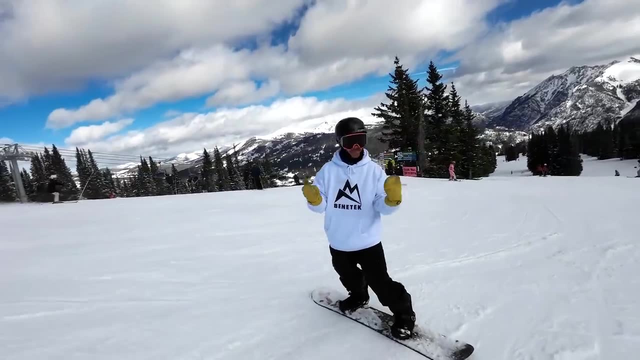 incorrectly. we should be able to be on the balls of our feet. toes are moving, yet we're still able to get this turn through the technique of knee steering. so I'm going to challenge you and myself to see if we can do that again. looking around, make sure it's a little busy, but I'm safe, I'm. 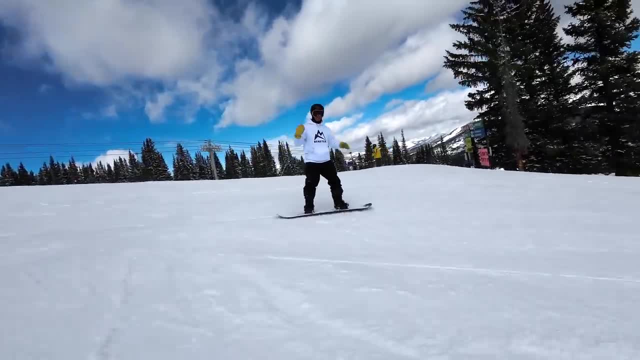 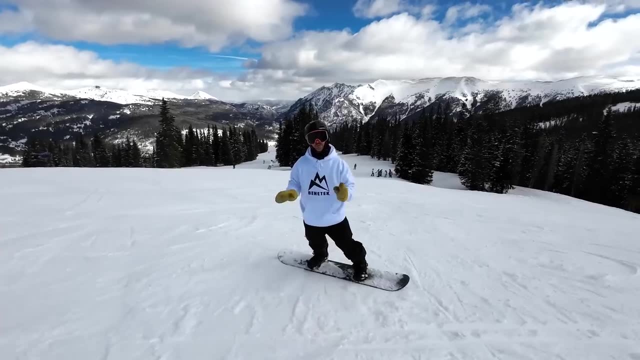 going to look around. I'm going to point my board down the fall line. one, one thousand two, I'm going to go a little faster. go around these guys. three, four, oh, that's interesting. so that is a fun little challenge to be able to get on the balls of your seat and to be able to wiggle your toes- just a. 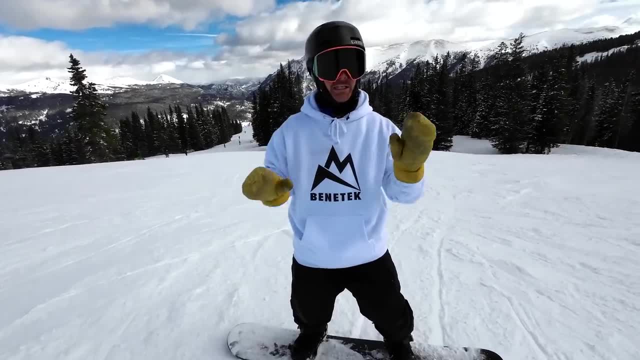 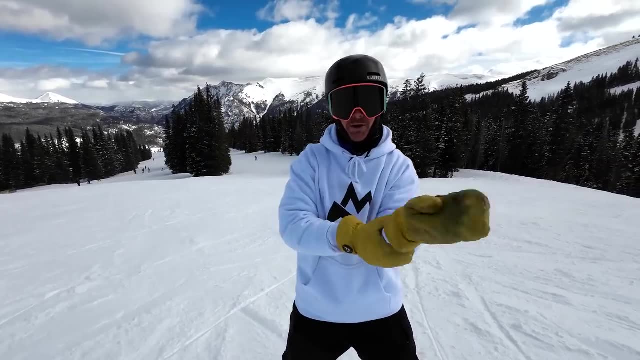 little bit. so now we're going to dive into a heel side turn, so the goal again is to be 60% of our weight in our lead foot. we're going to use knee steering. make sure that you're sinked down just a little bit so you have flexion in your knee, allowing your knee to move if you have your legs. 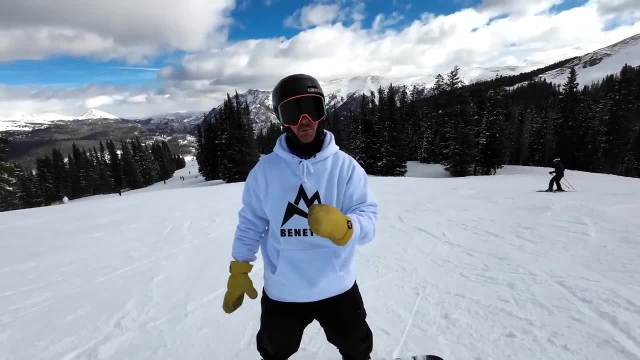 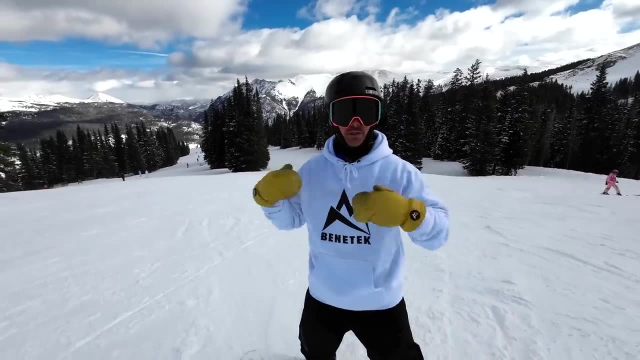 long. it's really hard to actually get that knee to shift or that femur to move in the way we need to, so we're going to point our board down the fall line. you can start from either heel side or toe side. for this example, I'm going to go heels or start. 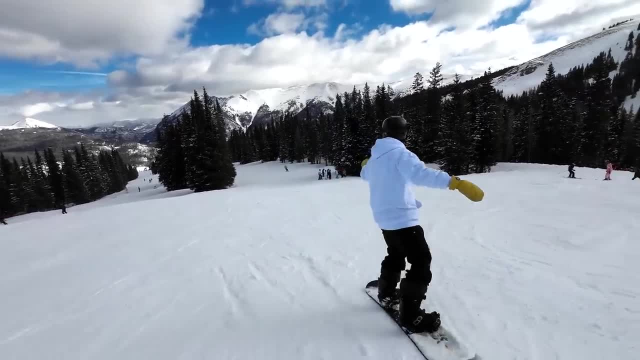 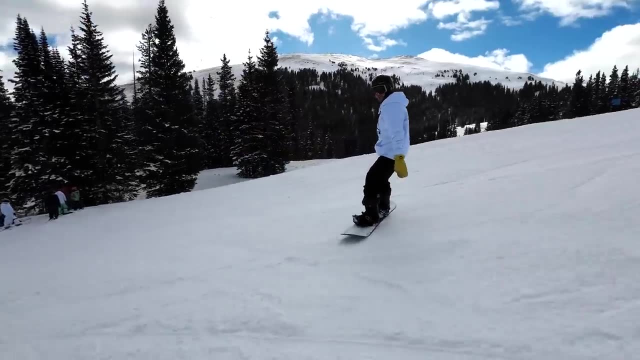 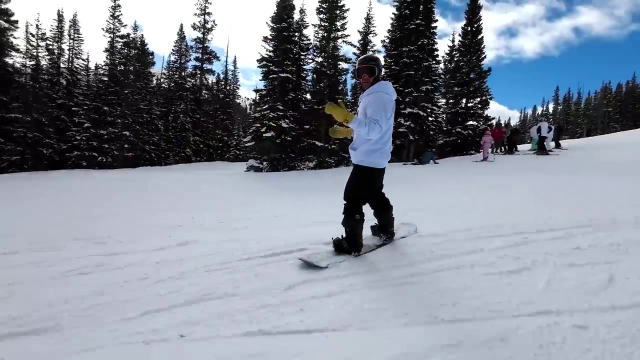 on my toes. so I'm going to point my board down the fall line one, one thousand, shift my weight forward, knee open. I'm going to do that again. we're going to point our board straight down the fall line one, one thousand, two, one thousand, knee and shift once again as I get my board to be across. 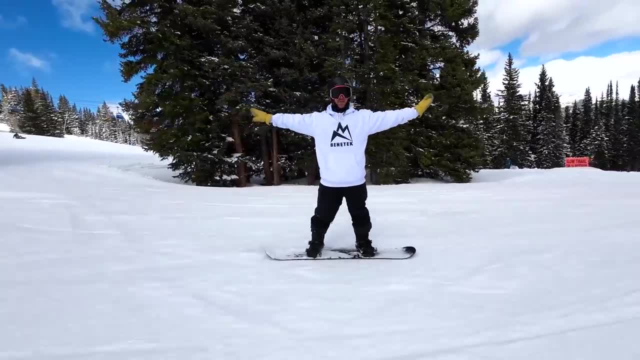 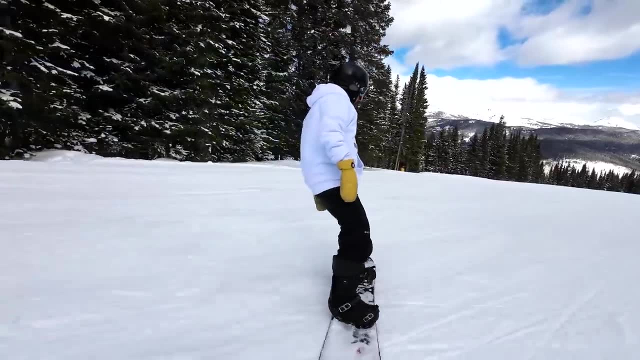 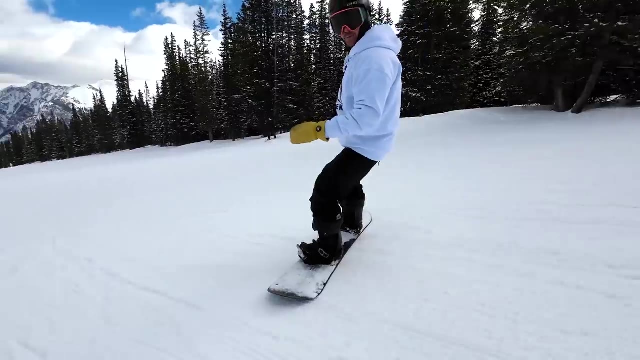 I'm lifting up my toes. now it's really flat. I can allow myself to think and process. one, one thousand two, one thousand three, one thousand four. I'm going to shift this knee and rotate. what I am looking for is to feel the outside of my foot actually helping the board pivot. notice that I'm. 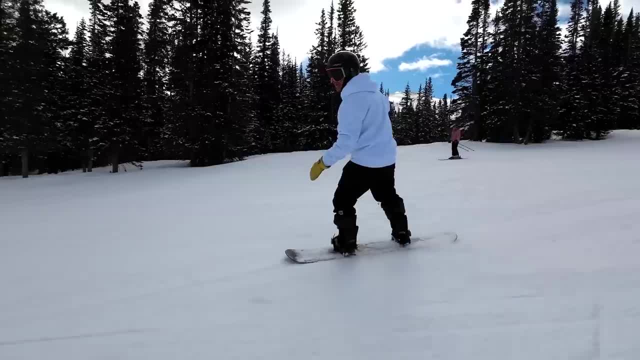 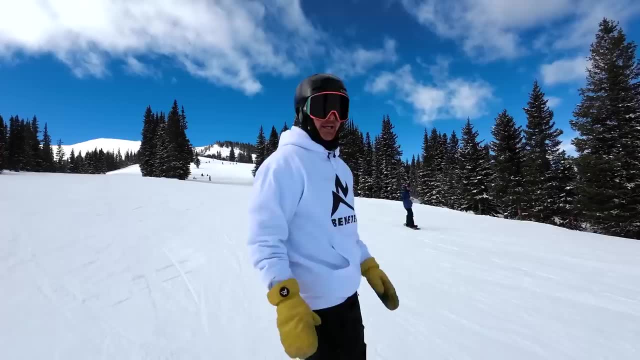 not back here trying to do it, because it doesn't work. as soon as I'm here, boom, very doable if you have the right technique. right here, right here, here, all right. now we're jumping into step three. ideally, what we're going to be doing is we are. 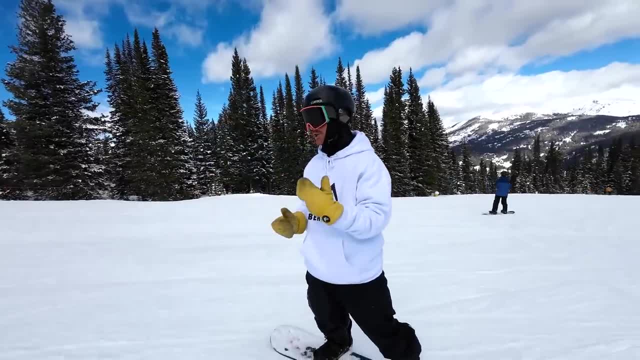 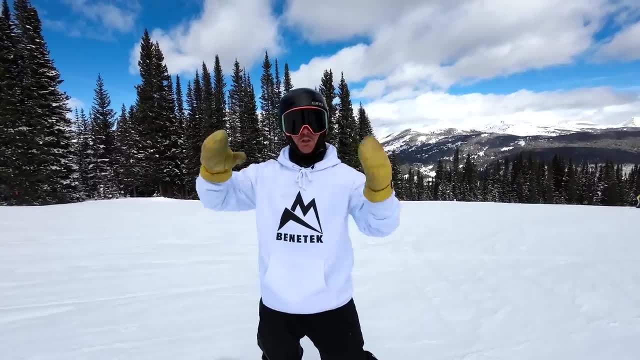 comfortable making a isolated heel side and isolated toe side turn, but we're now going to link them together. now the focus is still to point our board down the fall line between our turns so that we can process and feel everything, instead of just rapidly getting into it too quick. 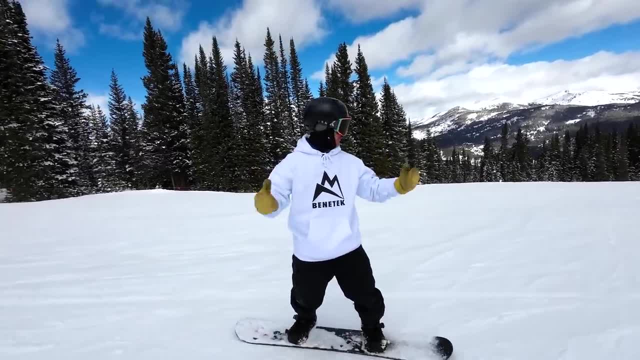 so we're going to point our board down the fall line. make a heel side tone, turn toes I turn. I'm going to talk to you throughout the video, so I am pointing my board down the fall line. one, one thousand, two thousand, I'm going to go heel side. 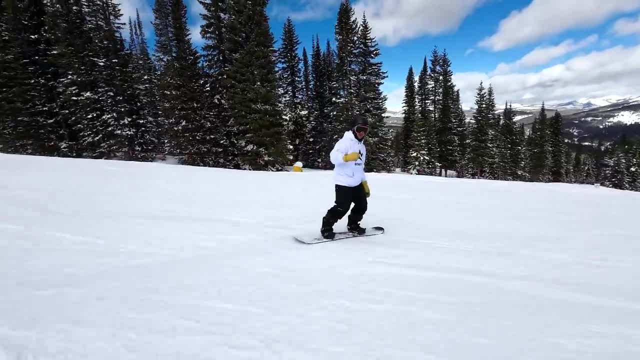 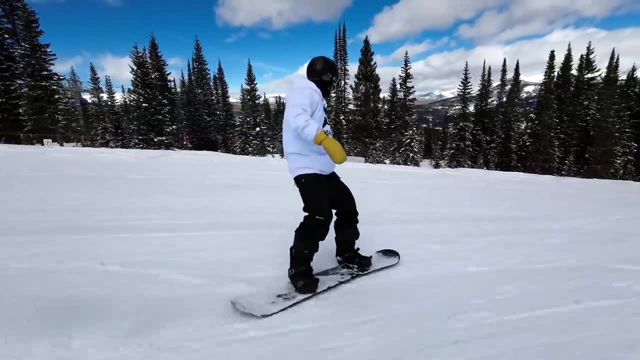 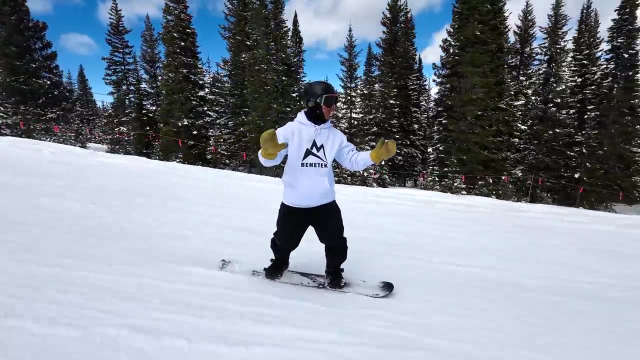 avoid this group. point my board down the fall line one one thousand two, one thousand knee steer. point my board down the fall line one one thousand two, one thousand knee steer. as I get more comfortable, I'm going to start minimizing the time between our turns so that 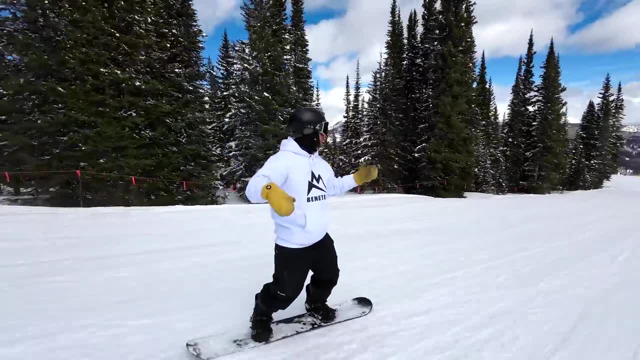 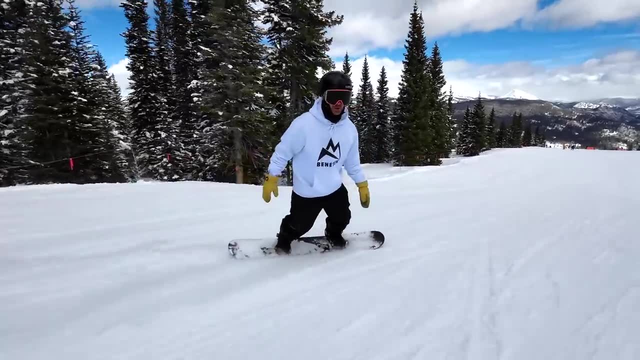 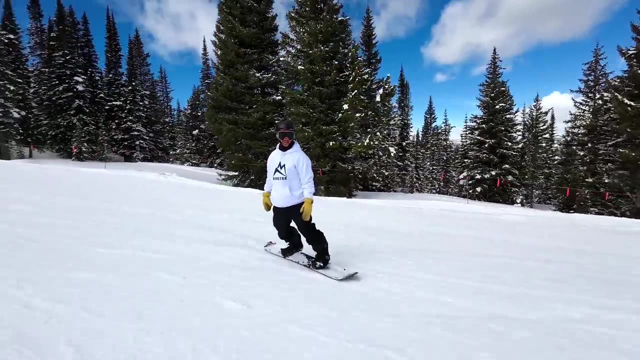 it can be one, one thousand, so I can make these sharper turns. so now it's going to start to look like this: I'm going to go heel side: one, one thousand, two, one thousand. oh, that was like one 1 000.. one 1 000, 1, 1 000, 1, 1 000.. now notice that I am on a very, very, very, very, very flat terrain. 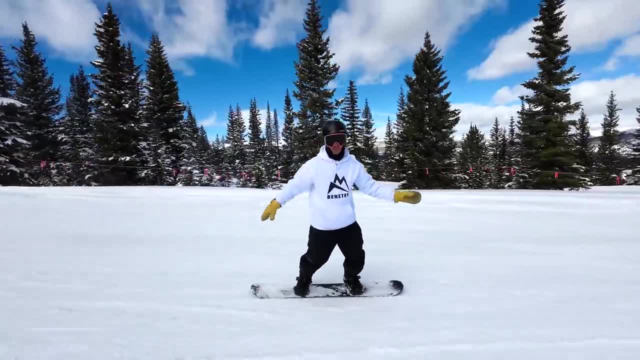 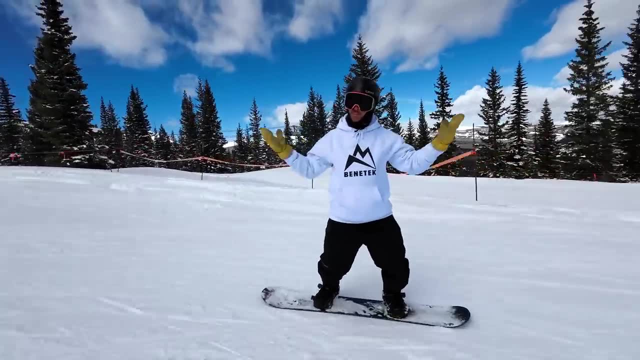 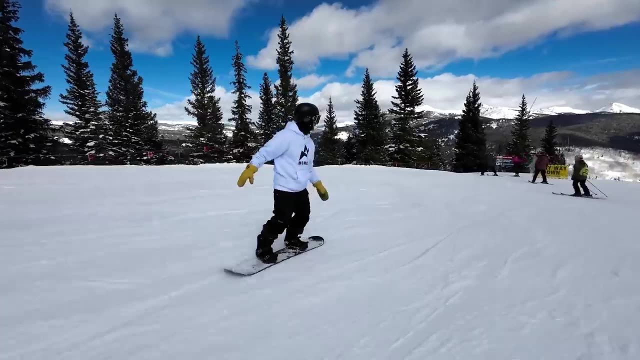 so I'm not able to close my turns, which means that I turned across the full line. anytime I turn across the fall line, I'm going to start slowing down. so these turns are a lot more open or a little bit a lot more elongated, allowing me to turn, but I'm able to keep up and manage my speed. 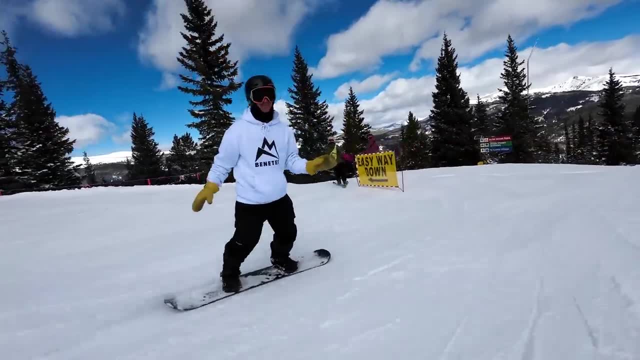 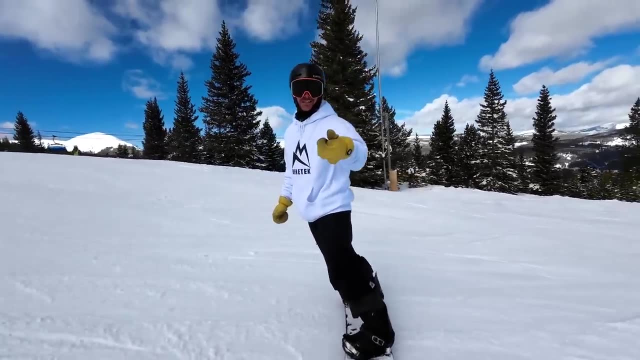 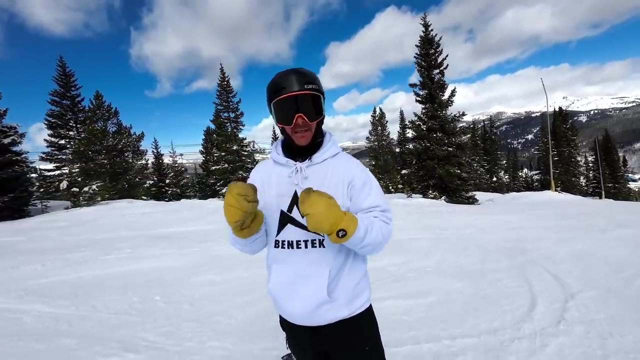 step number four be finding more appropriate terrain to challenge yourself. I have steeper terrain right here Now. I'm trying to minimize the time down fall line so that I don't accumulate too much speed. I am now shortening the time between my turns so that I can knee steer, knee steer, knee steer. 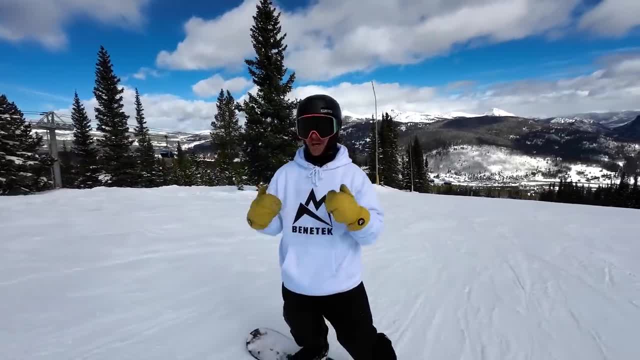 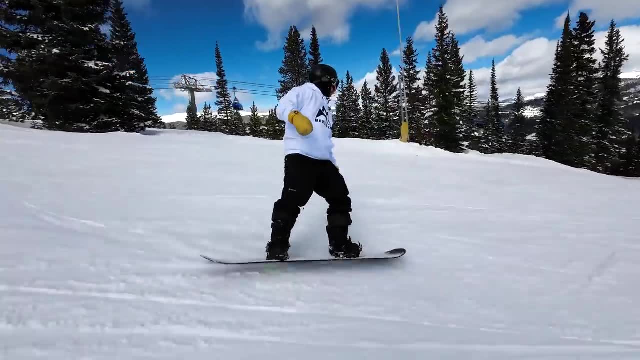 If you need to stay on step two, step three, step four for longer, definitely do so. So we're going to point our board down the fall line and I'm going to turn. I'm going to turn. Notice that my spine is upright. I'm not using my arms. Things are very smooth. 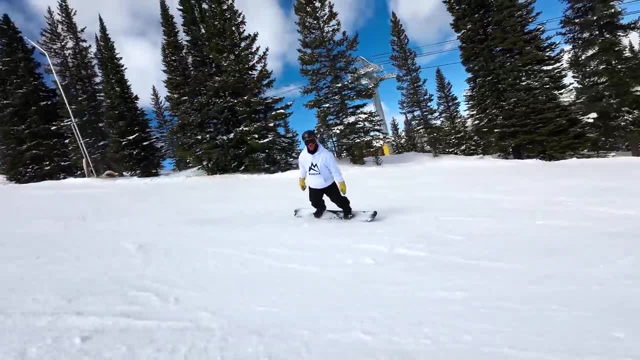 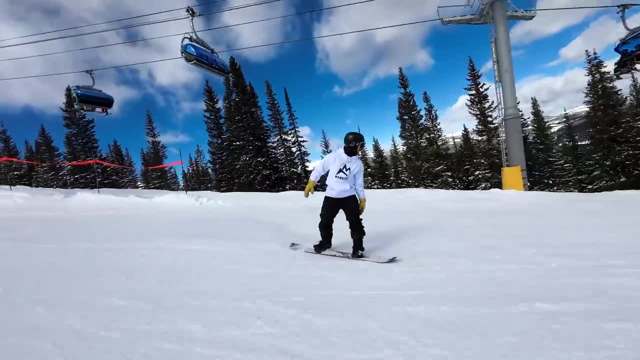 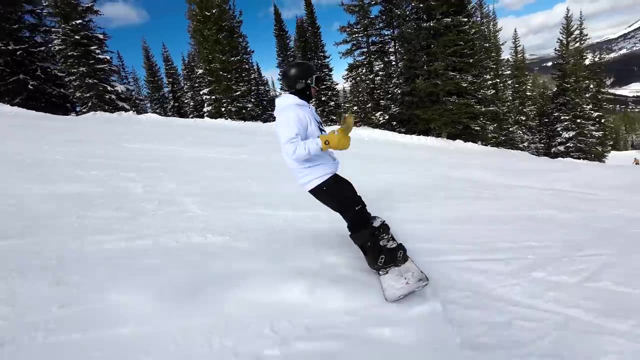 and I'm using my lower body. These turns are very controlled. I can make longer turns with less pressure or elongated pressure, or I can make them really quick Knee steer. Also, if you can hear it, which is my microphone- may or may not be picking it up- 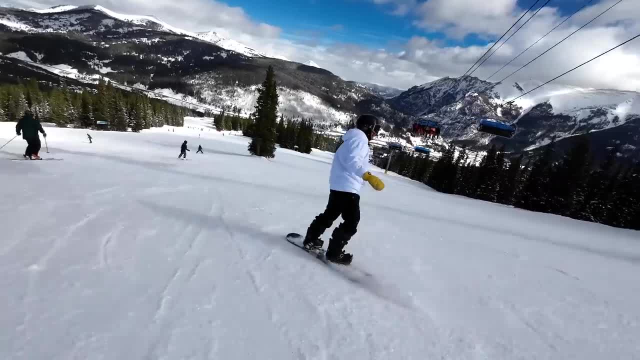 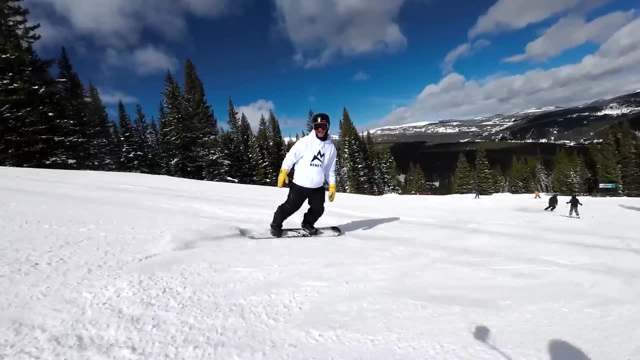 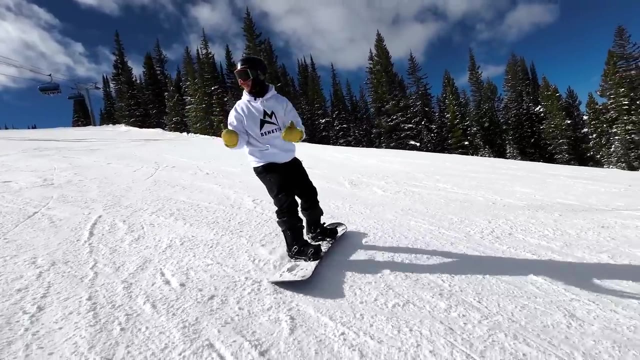 there's some really nice soft spots, but there's a lot of ice. Notice that my body is staying over my board and I'm not leaning into it so much. If I were to lean more into it I would chop out and fall like that because it's icy, it's steep or that it's gnarly. So I want to. 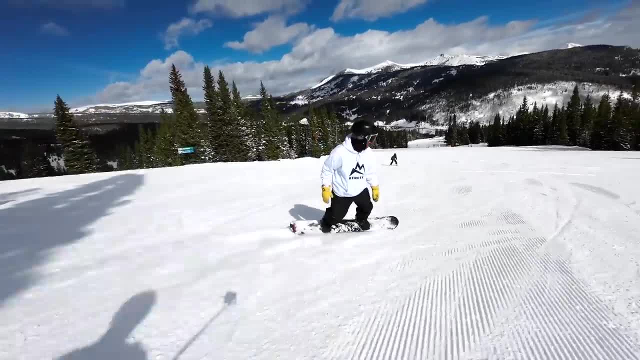 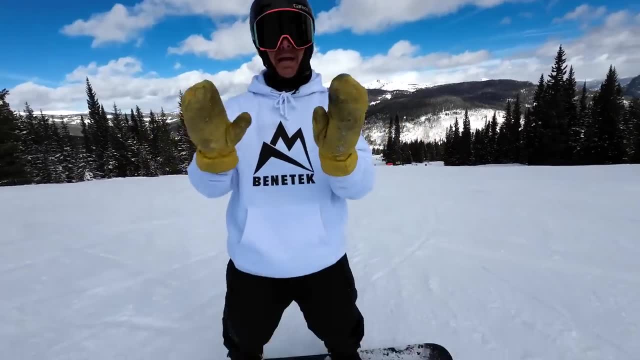 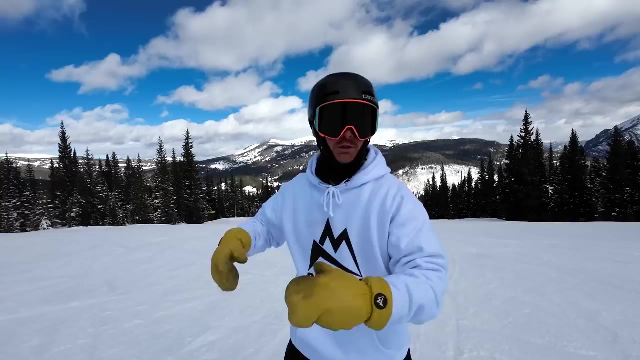 be able to keep my knees bent, making those turns just like this. Now you may be asking why or where do you use this technique? and I would say you use it 90% of the time, as long as you're not carving. If you're in the trees, you're in the moguls, you're on steep terrain.